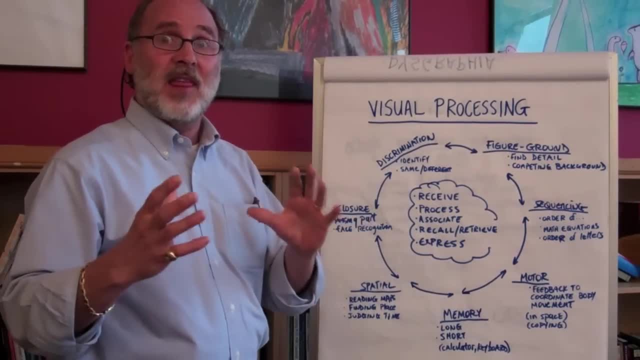 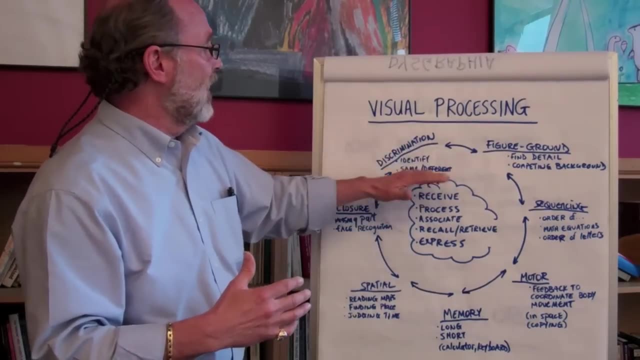 children will look at a letter and not be able to identify that letter as compared to another letter, or struggle to be able to tell a worry about another letter that I don't remember as tricky to –- same or different. And it's not just letters, it could be numbers, it could be. 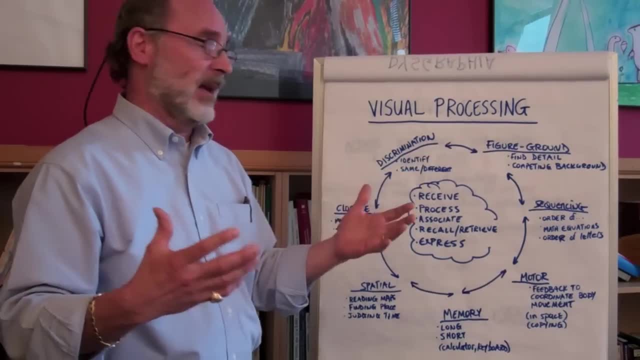 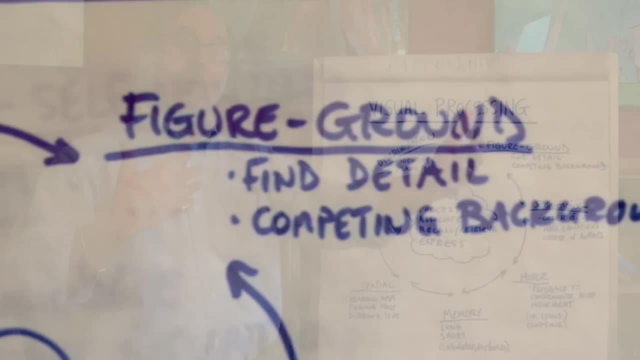 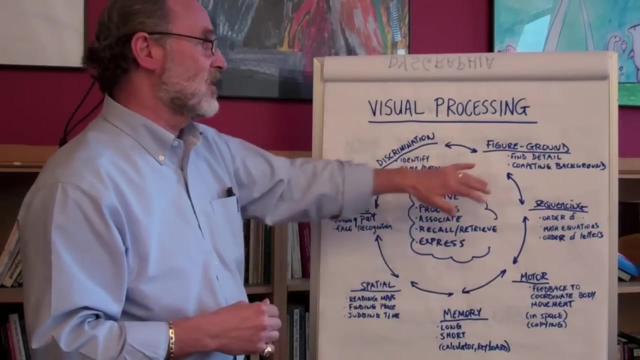 shapes. it could be any number of things where they have difficulty discriminating one thing versus another In terms of figure ground, meaning what's in front and what's in back, how things appear in space. individuals with learning disabilities often have difficulties finding details. So when you think about 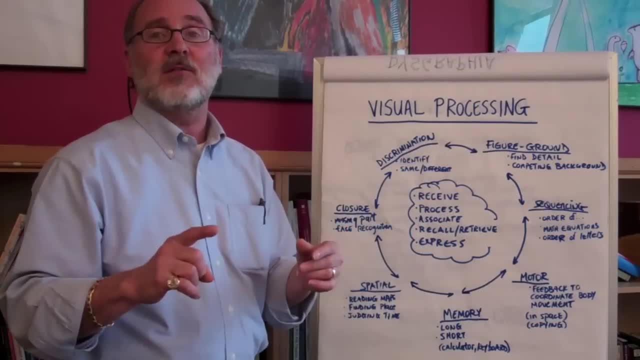 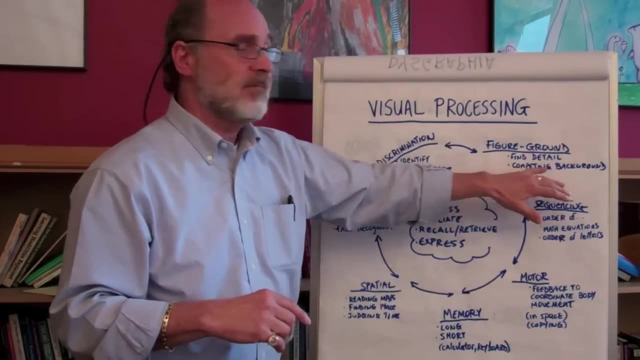 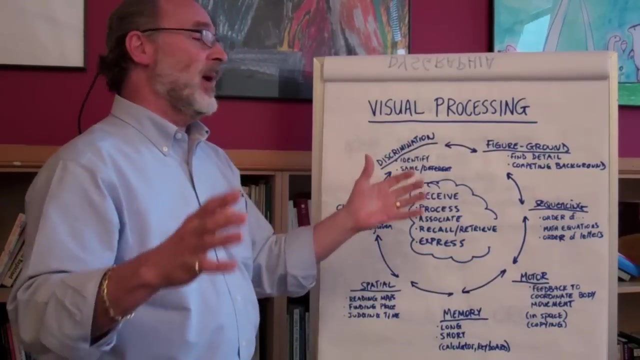 the Where's Waldo books very, very difficult for many students with learning disabilities if they struggle in this visual processing area And then being able to see things against the competing background. So that could be something very specific, or it could be looking at a page and picking something out from a. 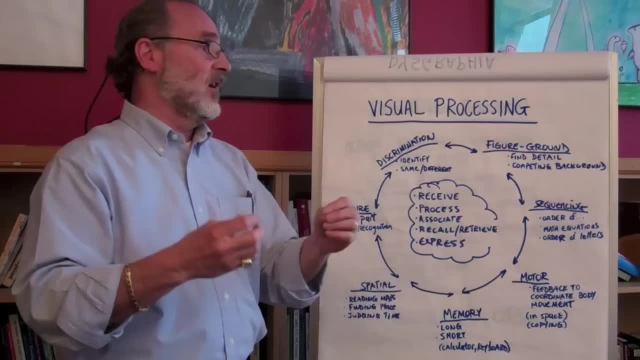 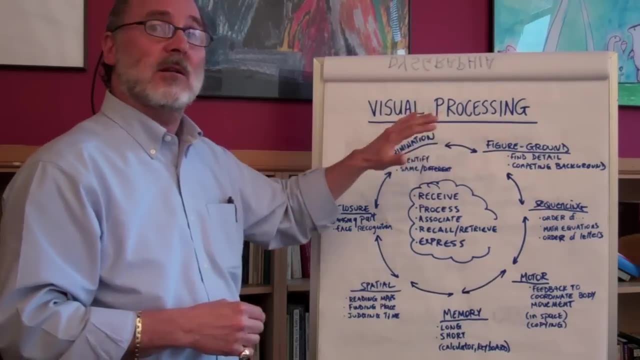 page. It could be a piece of text, it could be a piece of a graph, it could be a number on a chart. These are the kinds of figure ground difficulties that many students with visual processing difficulties have Sequencing. another area of difficulty for students with learning disabilities is the ability to 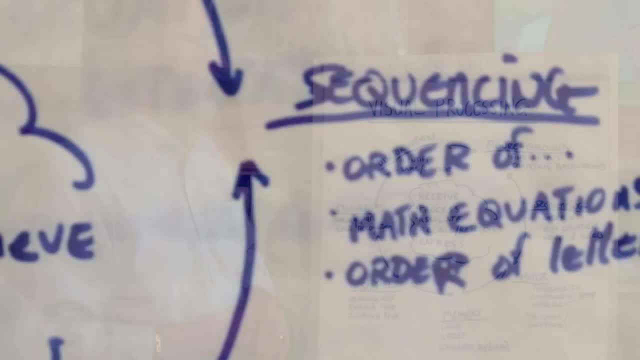 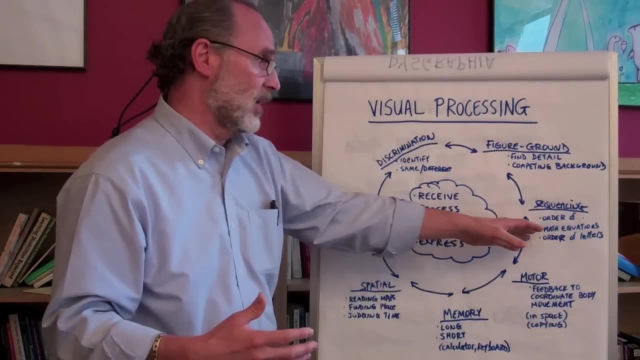 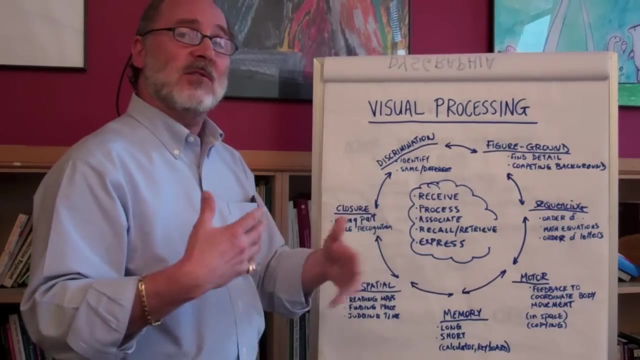 for students with learning disabilities who struggle in visual processing area, For example, the order of things how they appear. So, for example, in a math equation there may be numbers. in a sequence there may be the order of letters and words. Those kinds of sequences are often very difficult to discern and to remember and 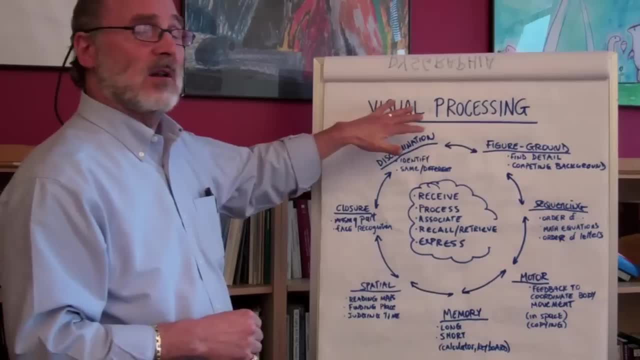 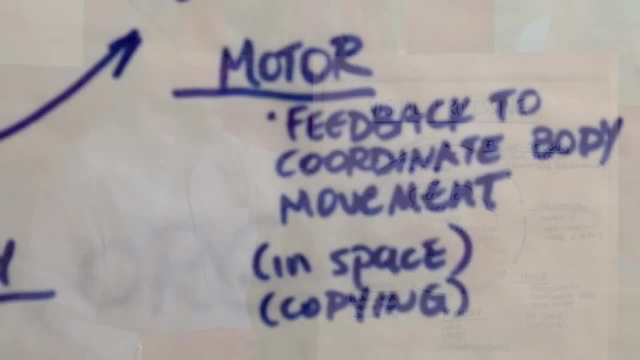 to recognize by students with learning disabilities who struggle in this visual processing area. In terms of motor skills, we have a lot of different methods to learn about the visual processing area, Motor processing or visual processing as it impacts motor functioning. very often, individuals with learning disabilities have difficulties because of the lack of 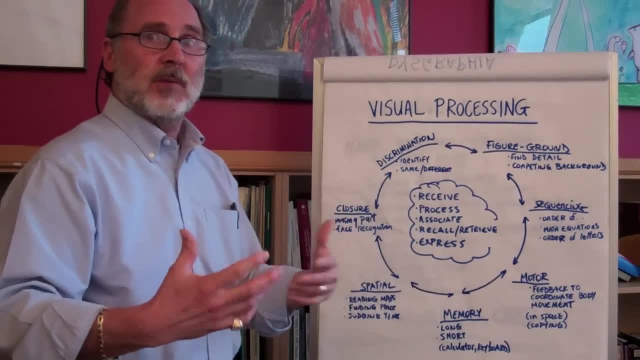 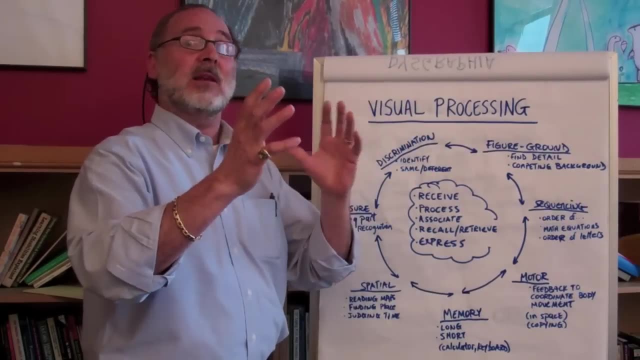 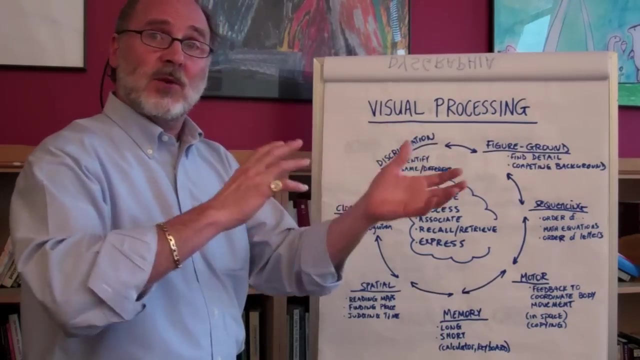 feedback that they need to coordinate body movements. So tossing a ball to them may be difficult for them to catch because they need to see that ball coming at them. They need to track the time with which it will take to get to them, How they move their body in response, What they need to do with their 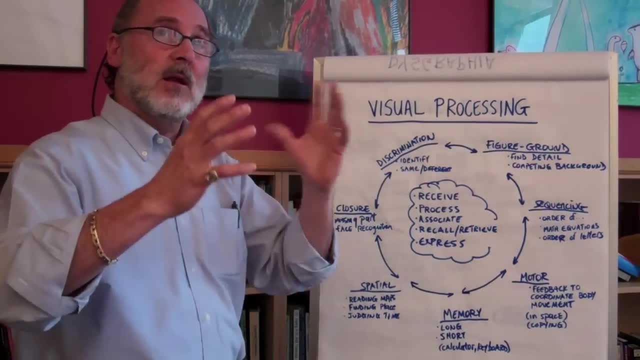 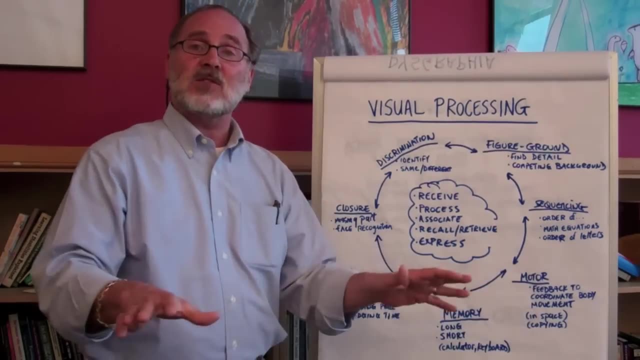 hands And so that visual processing and mapping and judging activity is really difficult for them. And it need not be just in space, it could also be on a flat surface, So, when they're copying, being able to coordinate some of those motor movements needed to be able to write and to draw.